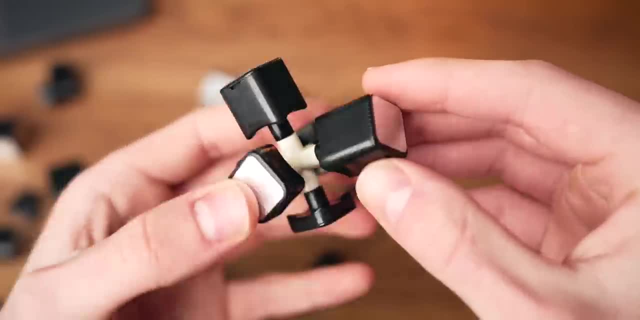 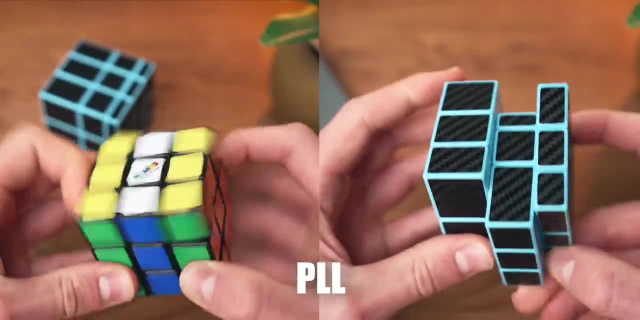 Each side has a different color. on a mirror blocks. Each side has a different height, so we can do the exact same steps on the mirror blocks as we would do on the Rubik's Cube, although just a bit slower, because turning a mirror blocks is weird. mirror blocks are actually a lot of fun. 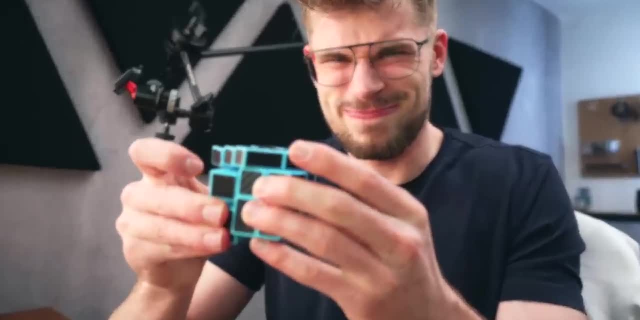 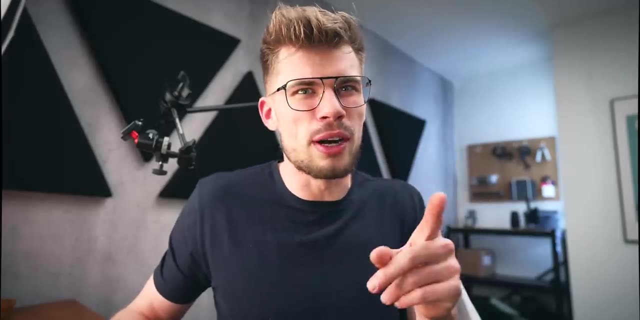 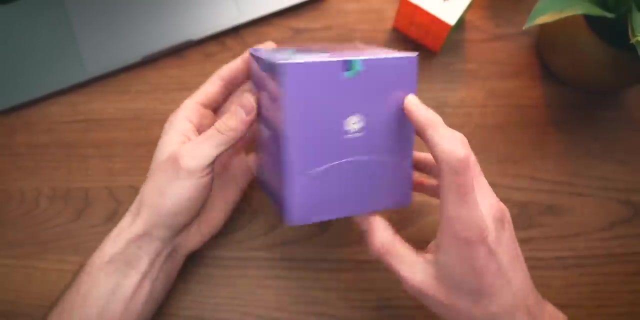 But they all share a similar problem, and That is why a little cube company by the name of GAN decided to disrupt the market by releasing their own mirror blocks: GAN mirror M. So here's the box and, funnily enough, even the box is a mirror. I mean, hi, this is not how you open a box. 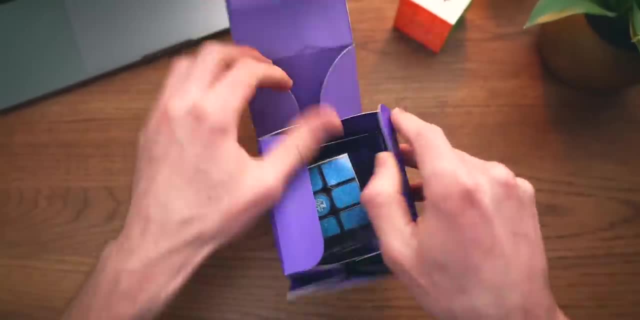 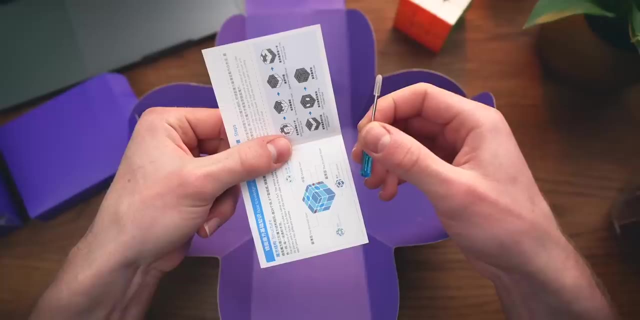 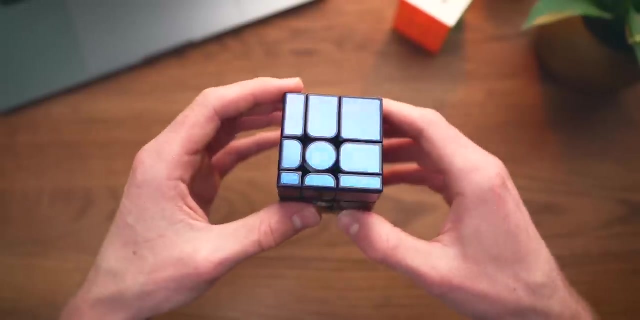 Okay, it isn't a mirror anymore. Here we go. Wow, Before we get to this beautiful piece of plastic, let's see what's in the box. That's not a lot. Wow, This actually looks really beautiful. So it isn't really a mirror. It's like this reflective purple color, but I'm let's do some first turns. 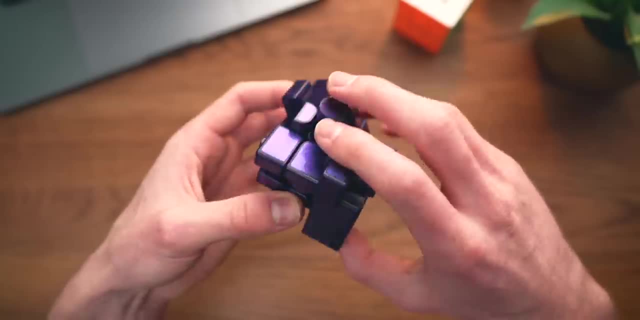 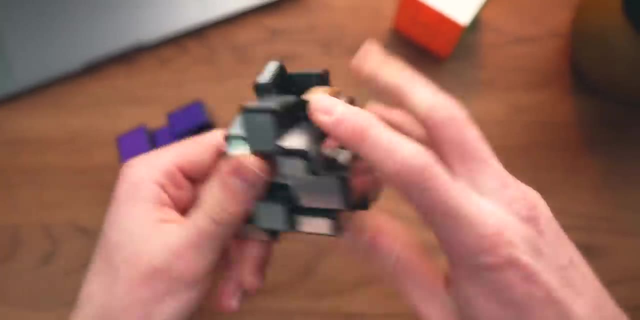 So it's obviously really awkward for me to be turning a mirror blocks because it's constantly changing shapes, But I can definitely tell straight away that it turns better than this guy right here. So what you need to know about this puzzle is that, first of all, it is magnetic, so it snaps into place after each. 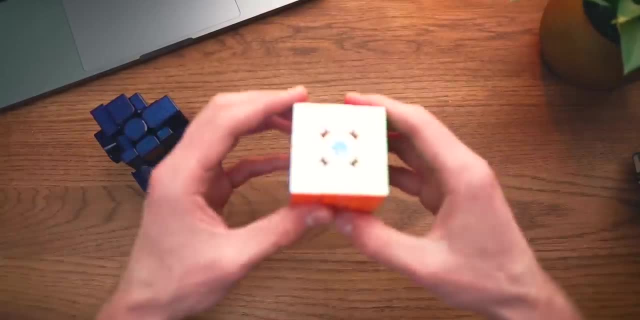 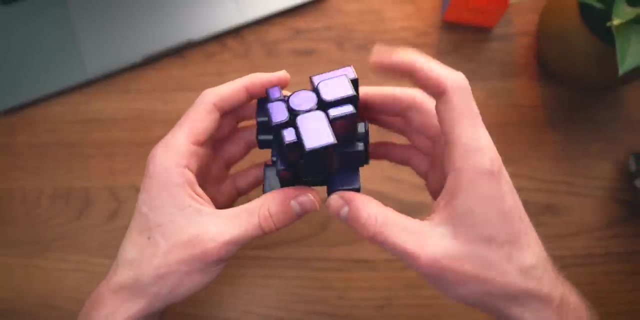 Turn aside from that. it is really built like a speed cube. I mean, this is a GAN flagship speed cube. I Could just spam TPS on that, but I'm not used to this, so I won't be doing that anytime soon. Yeah, I guess that's all I can. I may not be a mirror blocks expert. 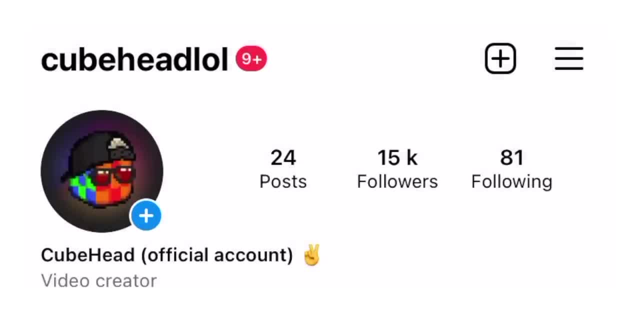 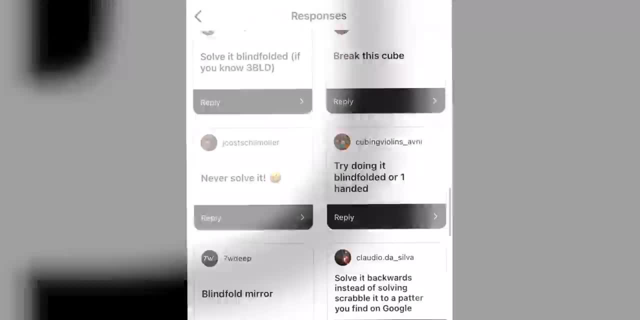 But I will be at the end of this video because I asked you guys on my Instagram- by the way, please follow- I post epic pictures. I asked for challenges. I could do with the GAN mirror M and from your answers I chose 10 of the most epic challenges. 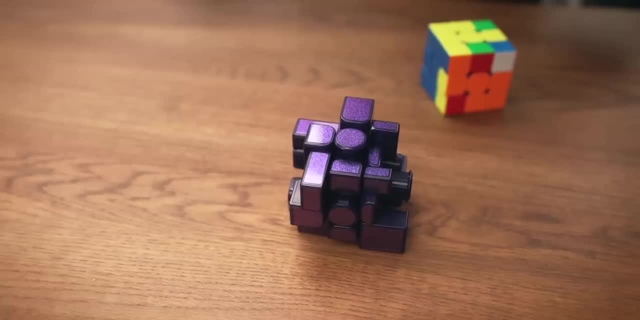 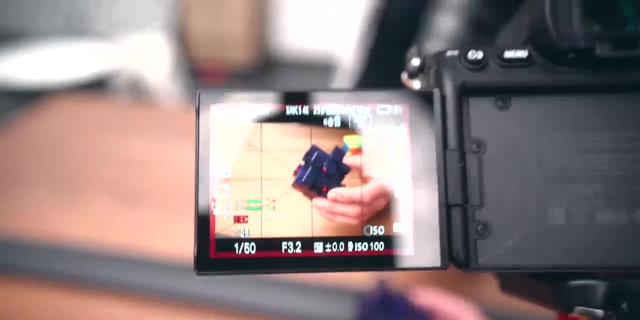 The first one is solve while only looking through a mirror. This shot looks pretty normal, right, but it is actually the reflection of my mirror. What so? if I only look through the viewfinder of this camera, I can only see the reflection of the puzzle and not actually the puzzle itself. Oh, this is so weird. 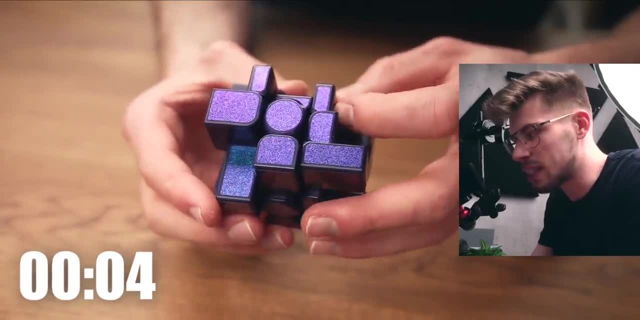 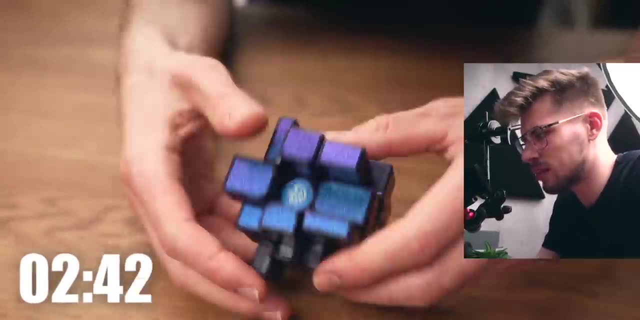 So I want to. I want to put this one down, But it feels like it's going up, which is super weird. I haven't done a single turn. Yeah, remember I went over the different steps to solve the Rubik's Cube in the beginning of this video. 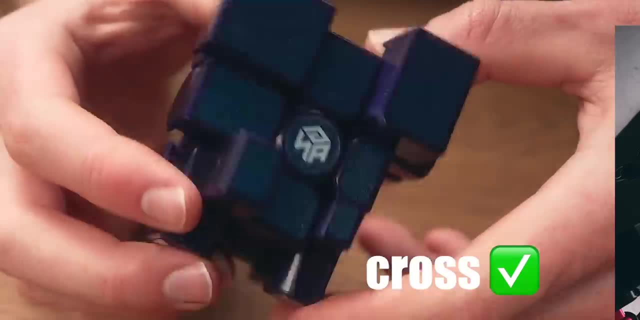 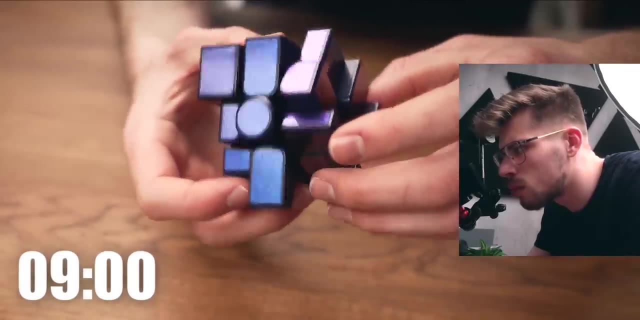 well, after seven minutes I finished the first step and At this point I was starting to be able to link the movements of my hand through what I saw in the mirror. But even then I was often touching pieces just to double-check I was actually solving the right piece. 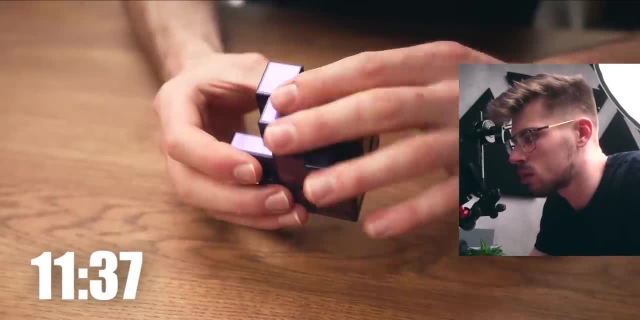 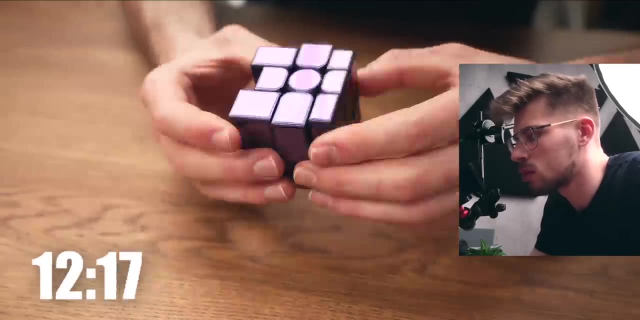 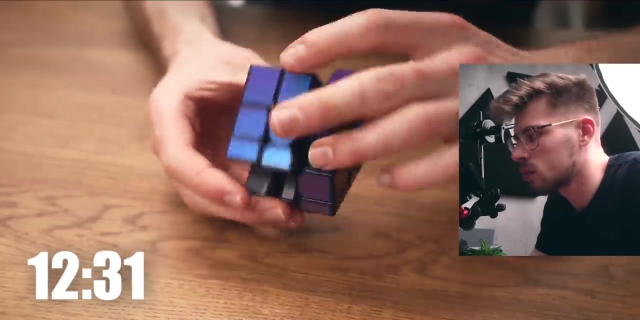 When I got to the last layer of the soul, things were a bit easier, because it wasn't much about tracking pieces at this point, but more about doing algorithms from the right angle. and Then, after twelve and a half minutes, I did my last algorithm, which is kind of crazy, because the first four pieces took me seven minutes to solve. 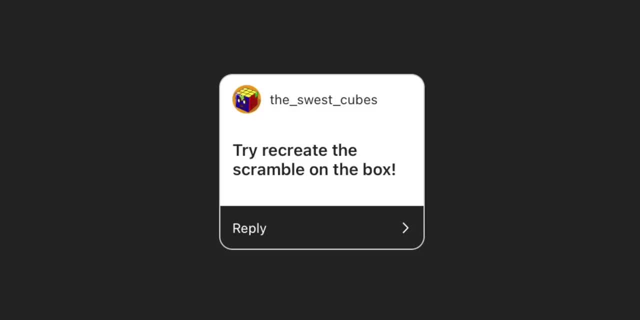 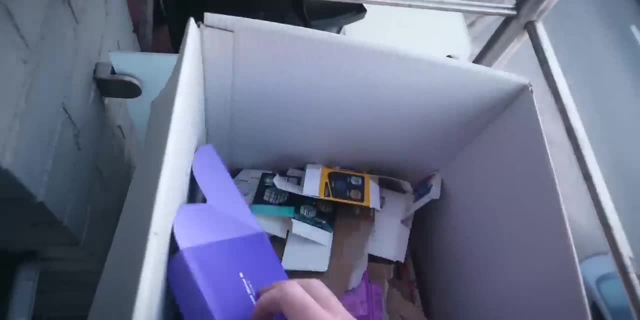 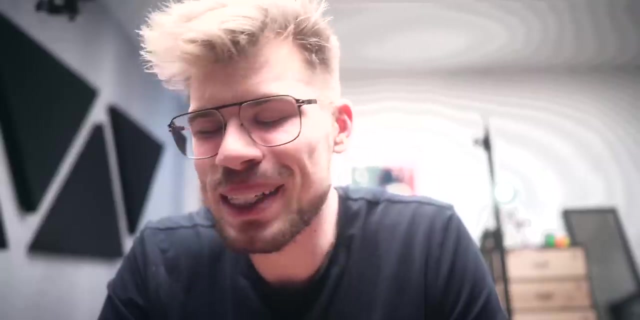 The rest of the cube, just five Recreate, the scramble on the box. I actually threw away the box, So we gotta find it back together There. it is okay. so we got a recreate that. I Seriously spent 20 minutes on this but this is the closest I'm gonna get. but then I remember that the underscore Swiss underscore cubes. 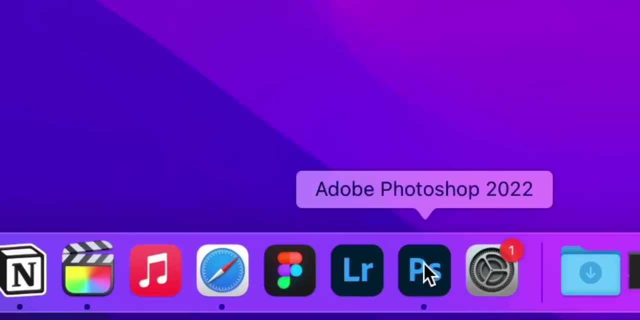 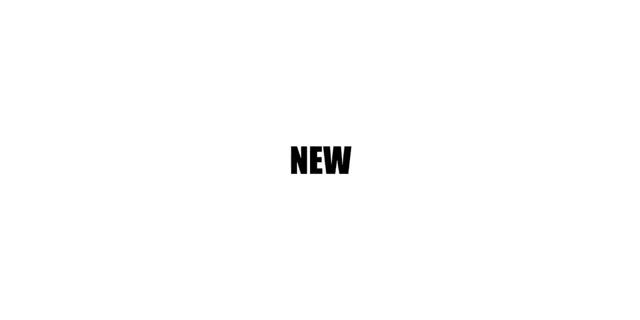 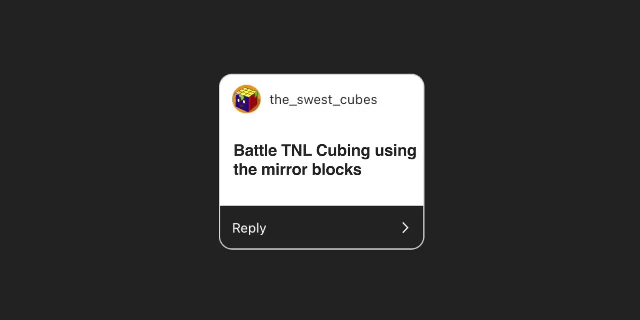 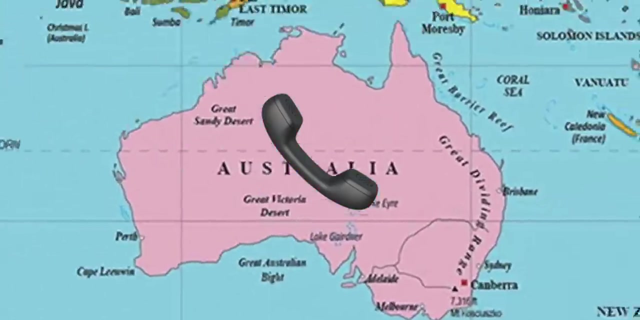 They didn't give me any rules, So I actually had never, ever seen the dime Battle TNL cubic using the mirror blocks. I'm even waking up early for this video. Your Tom, do you have the new GAN Miracube? because people are asking us to race, Uh yeah. 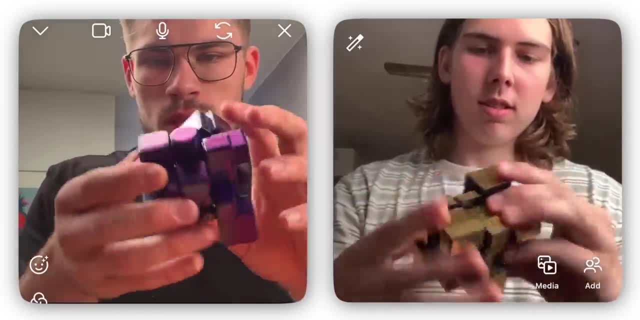 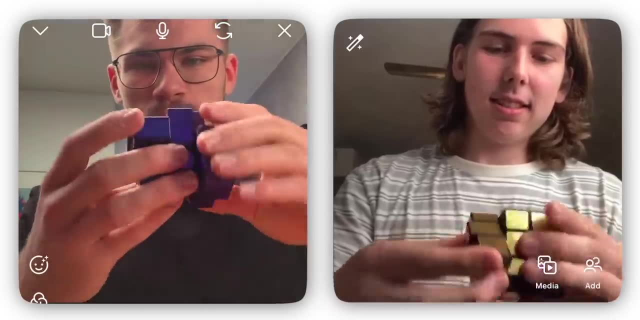 All right, let's do it. He's Tom had spent more time in the art of mirror block. this ought to be a difficult challenge. what's happening? i cannot solve it. i'm on the pll, but when he was nearly there i suddenly got a boost and oh no, tom is locking up. what is he doing? 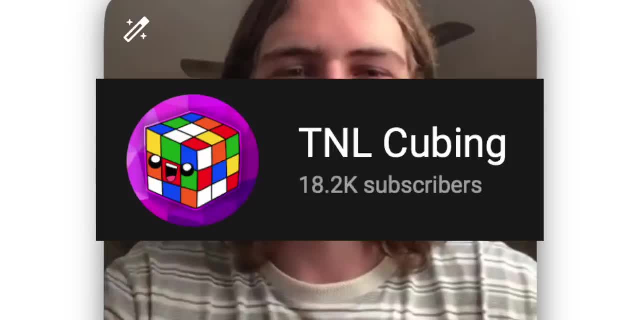 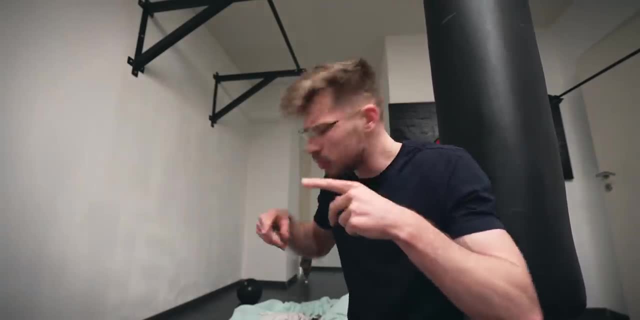 all right, it seems like i won what goes up. the tiny loser cubing. i finished like a minute. solve it while hanging upside down. i can do this challenge because i have a pull-up bar. i also put some blankets on the ground because, you know, if i fall down, i might, i might actually die. 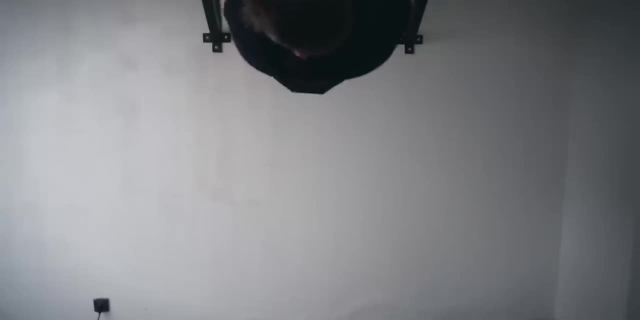 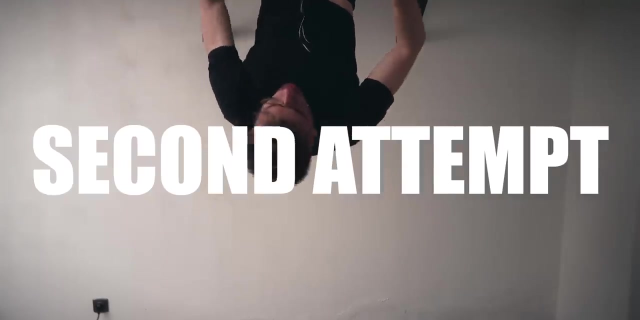 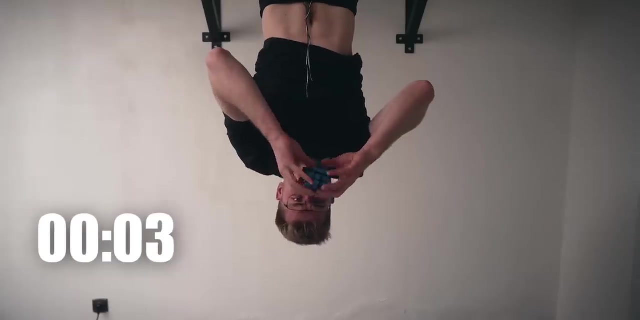 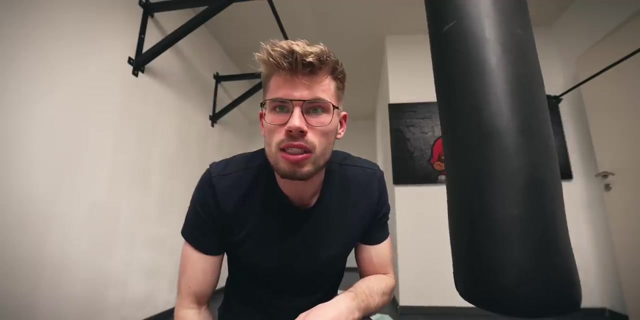 oh, this is so scary. okay, let's just go, let's just go. oh my god, oh my god, i'm actually gonna die. i cannot do this. i cannot do this. what the hell? oh, my head is so red, i thought i was gonna die. i couldn't hang upside down for a few minutes, so i just did. 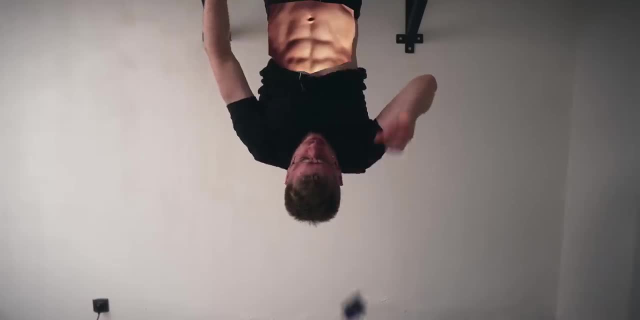 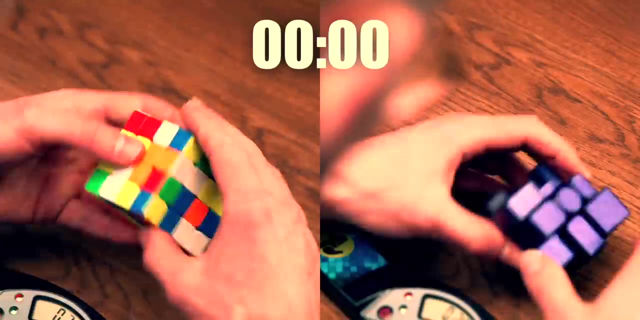 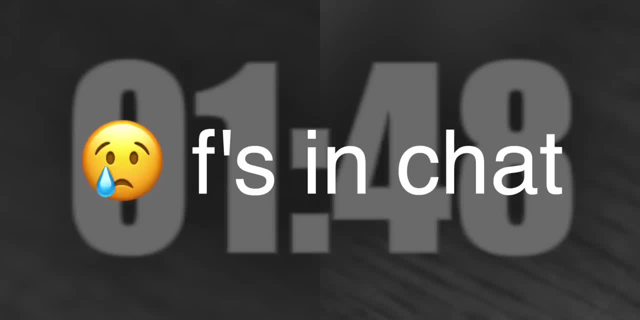 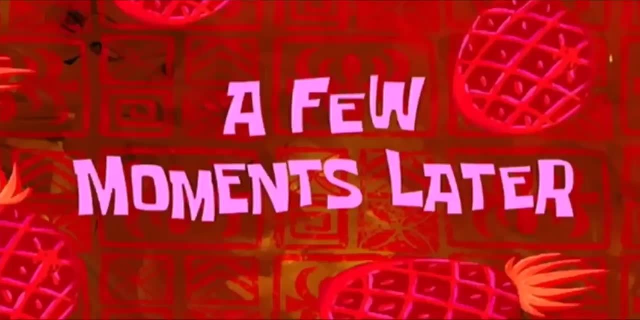 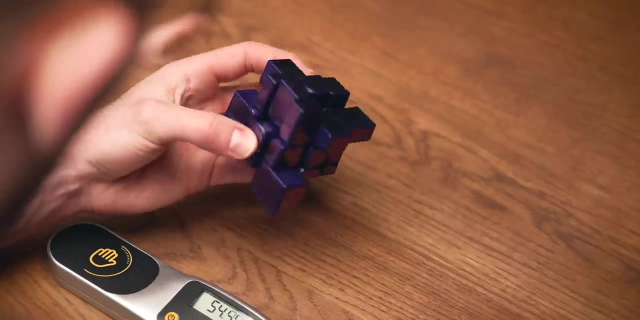 a lot slower. that means one-handed, but phil doesn't know how to form sentences. i don't think this one will be that hard, though. a few moments later. when do i start? a little later, oh my god, much, much later. what the hell corner twist? do i need to do this one-handed? 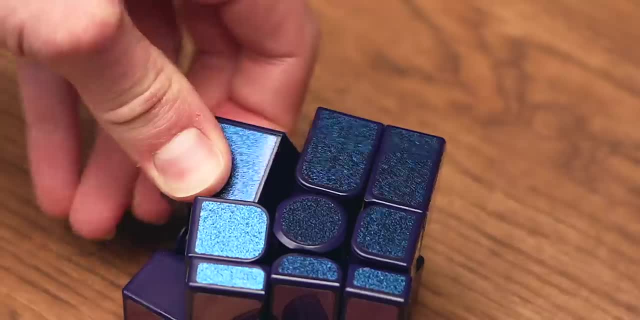 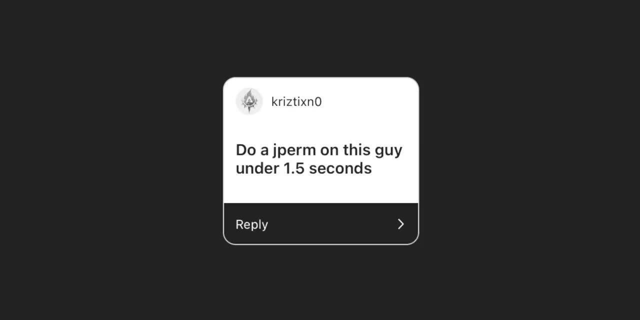 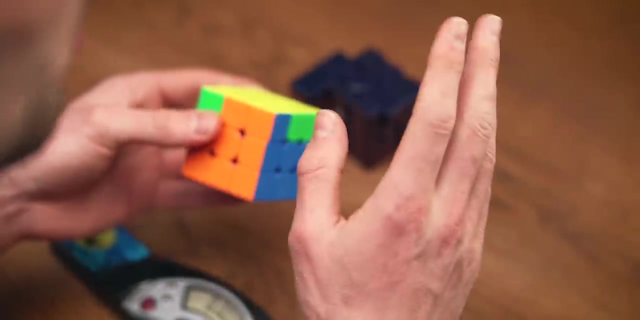 as well. i'm gonna break this puzzle. okay, why is this the most frustrating video to make? do a jperm on this guy under 1.5 seconds, this one goes out to jperm himself because he just reached 1 million subscribers. that's insane. if you for some reason don't know, jperm is an algorithm to solve this. 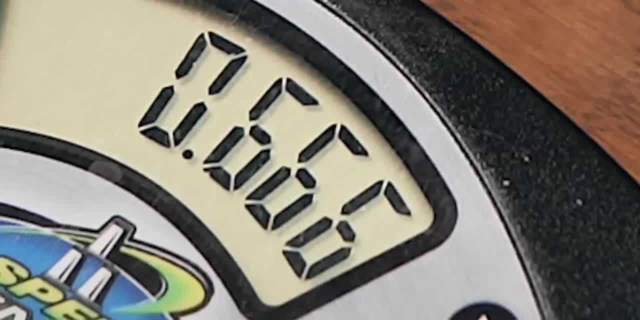 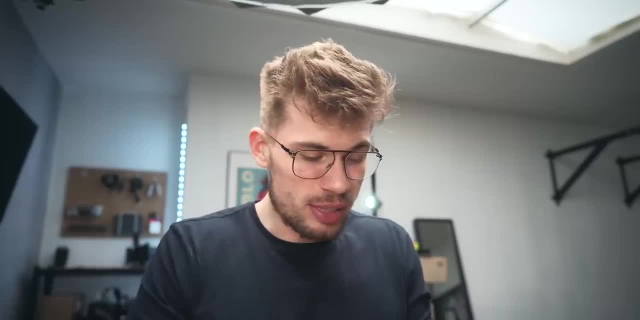 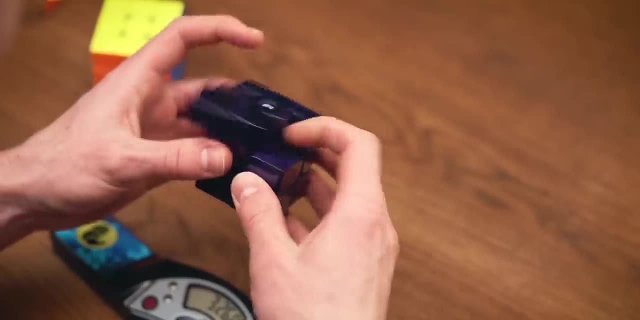 case and it goes like this: it's really fast on a normal cube, but uh, yeah, on this guy it's gonna be a bit more tough. except 1.5 is the goal, let's go. can we find a layer that's actually easier to finger trick? the small layer is definitely. 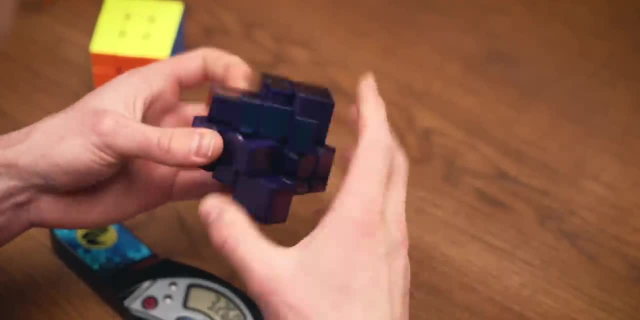 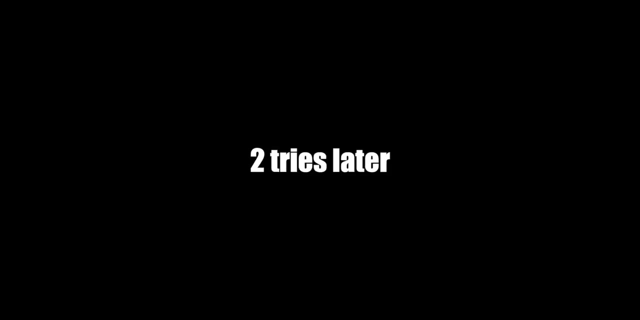 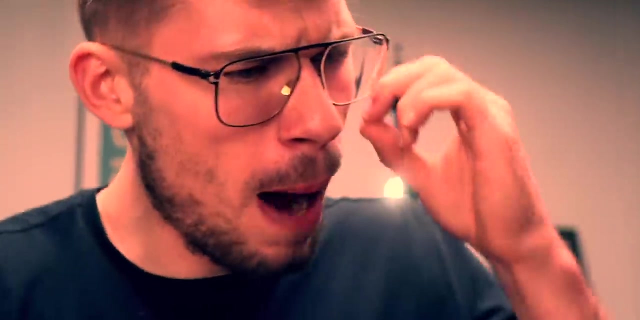 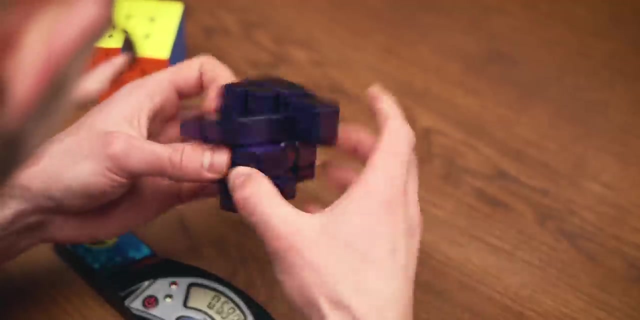 not it, maybe the biggest layers. yeah, that's definitely better. oh, this is gonna be a lot of work, but i'm gonna do it. i'm gonna be the one guys we can do even faster though. oh, let's go solve it blindfolded by just feeling the pieces. my